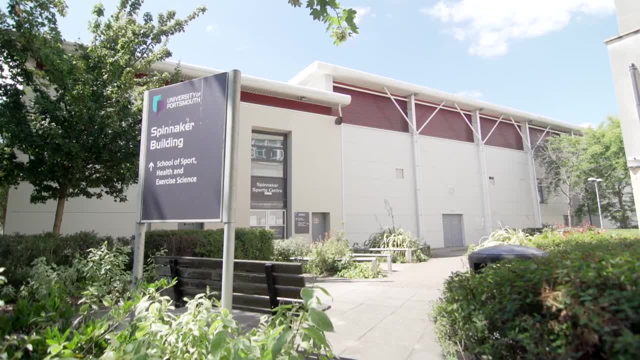 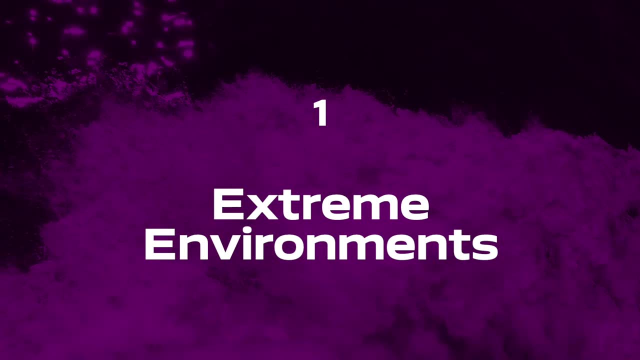 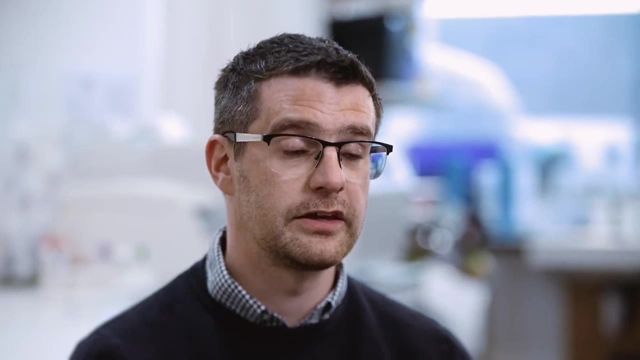 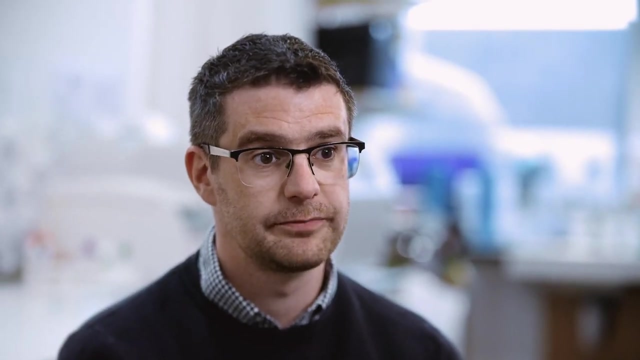 Our research spans the broader area of sport, health and exercise. We have three research themes. The first is Extreme Environments: It focuses on the selection, preparation and protection of those who enter extreme environments. The second is Physical Activity: Health and Rehabilitation. So we focus on clinical and also non-clinical conditions and also how. 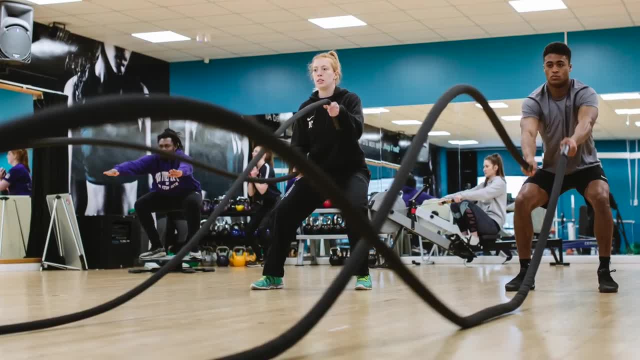 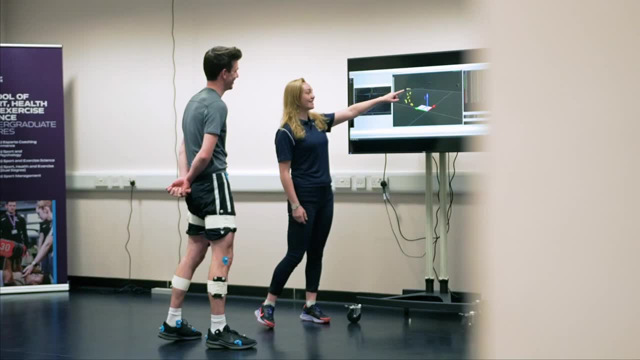 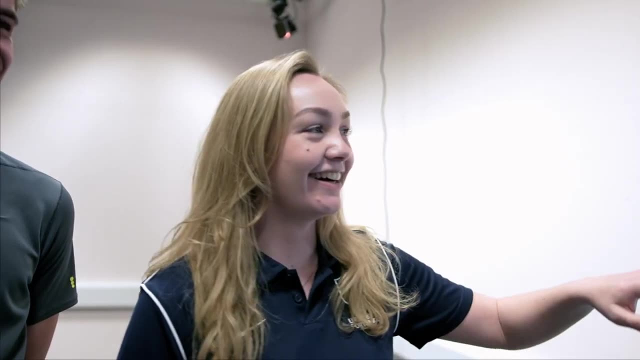 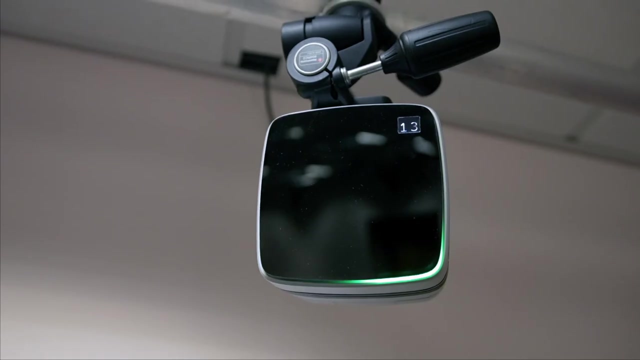 physical activity can help improve the lives of people. Our third and final theme, Individual, Occupational and Organisational Performance, looks to see how we can improve the performance of individuals, organisations and teams. The facilities that I use at the university is our biomechanics lab. The types of equipment that we use is a 3D camera system, which allows 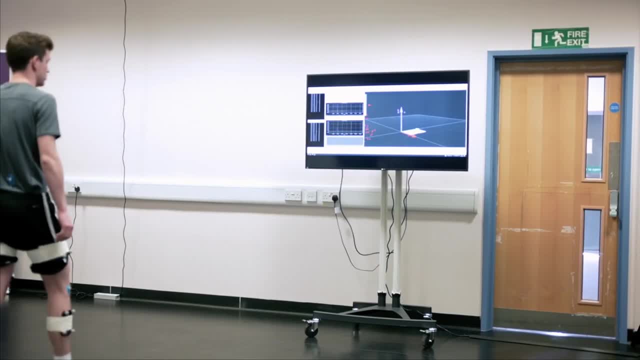 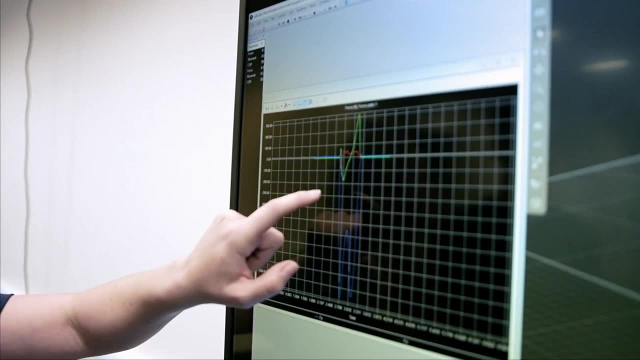 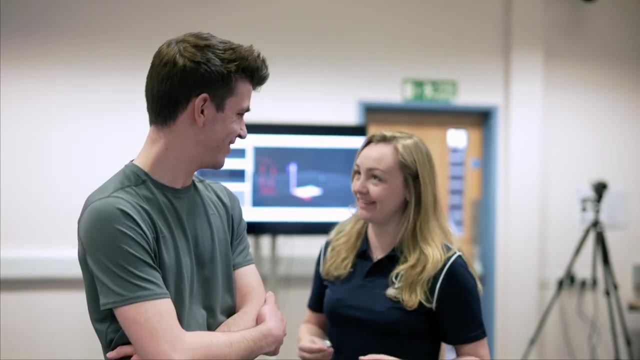 us to put markers on an individual and track their movement in 3D so we can really see their movement in detail. We also use force platforms to have a look at the ground reaction forces and also EMG as well, which is electromyography, which allows us to look at muscle activity. 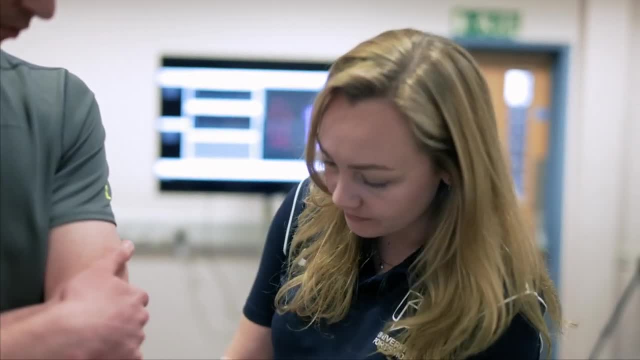 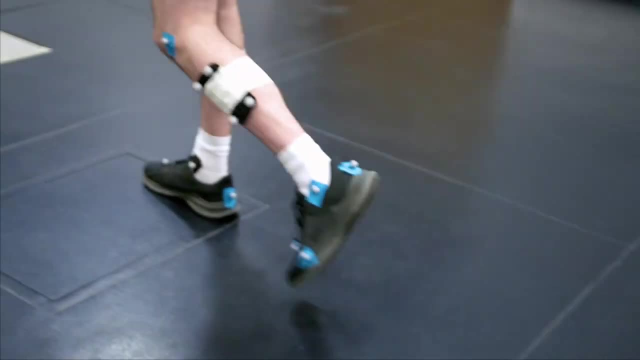 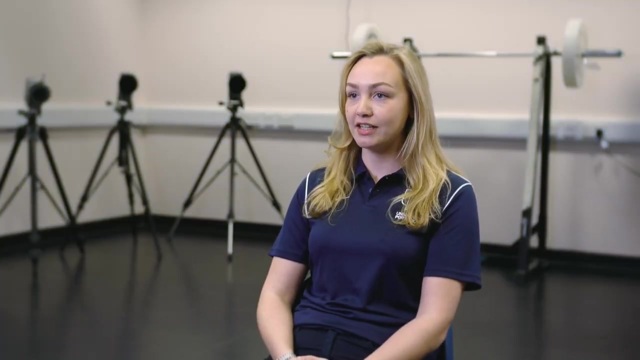 and we can track that through different rehabilitation processes. So the outcomes that I've seen from my research has been improvements in walking speed, for example, which we know is one of the high outcomes of quality of life for individuals who live with stroke. In sort of the preliminary research that we've had a look at, we've 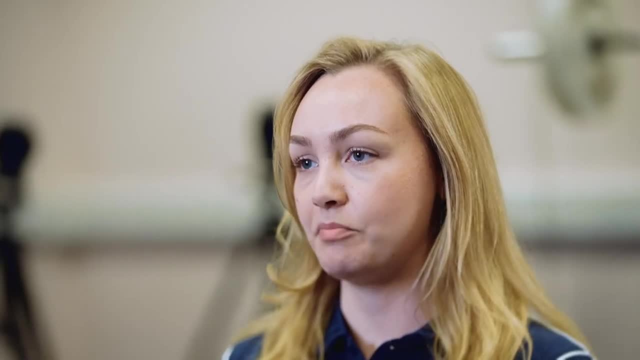 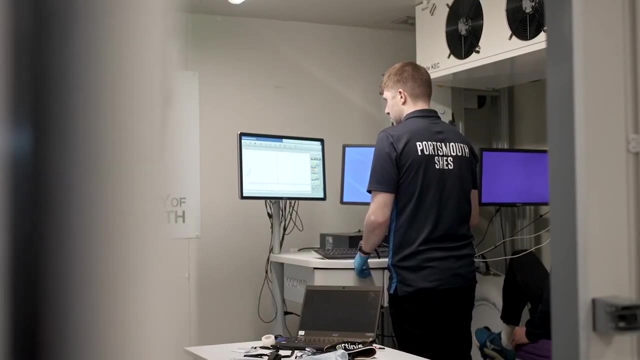 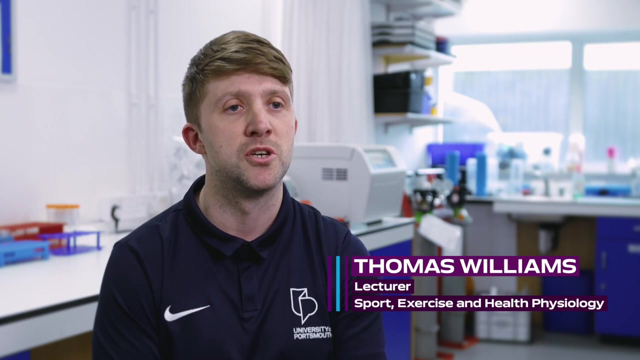 found that it's looking positive in terms of using different robotic rehabilitations to improve functional outcomes of individuals with stroke. I'm based with the Extreme Environments group and they've built a reputation over many years of looking at the physiological responses to all of our different extreme environments. 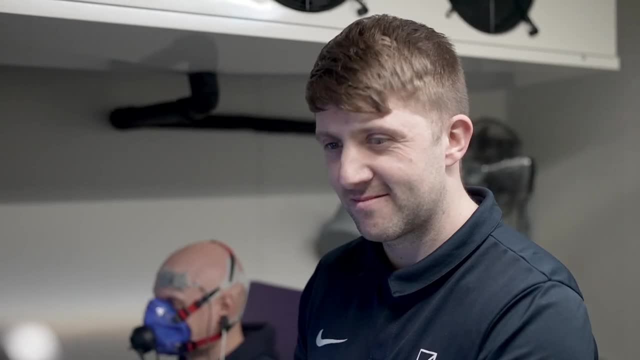 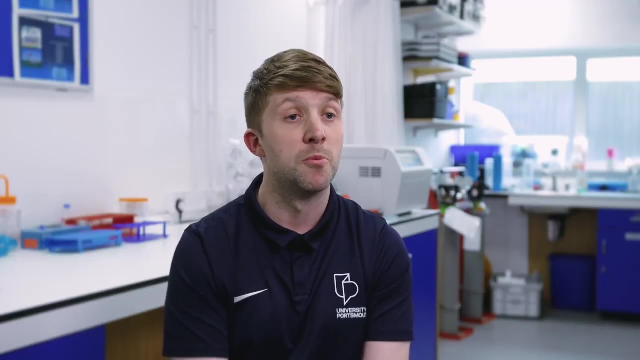 so our heat, our cold and our hypoxia, We can effectively recreate any environment that you would come across on earth. So we've got a heat chamber that can go up to a around about 50 degrees. We've got a cold chamber that can go down to about minus 20. 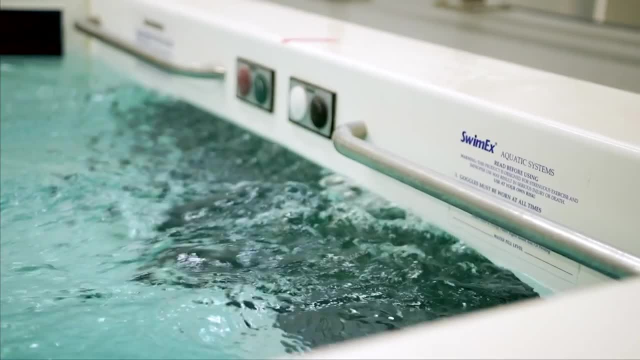 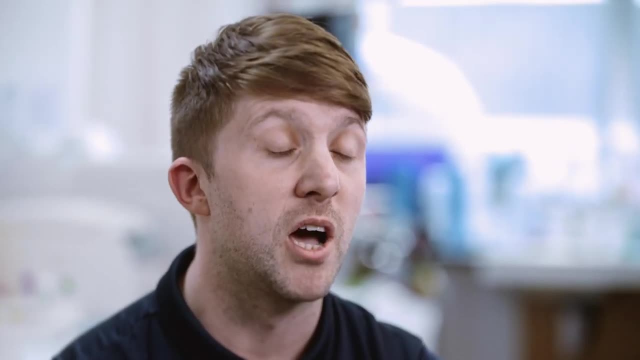 and then we also have another environmental chamber that contains a flume, And then all three of those chambers can create a hypoxic environment or simulate altitude, So we can go anywhere from sea level to around about 8,000 metres. So we could effectively put.